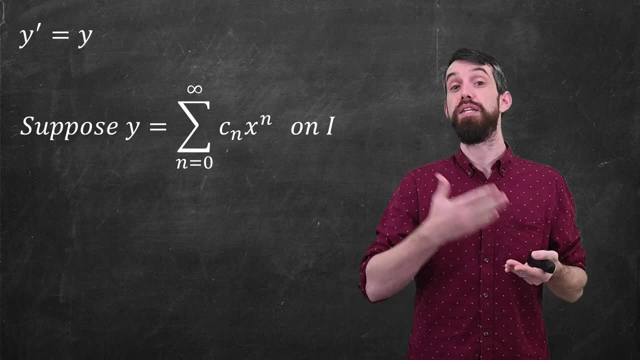 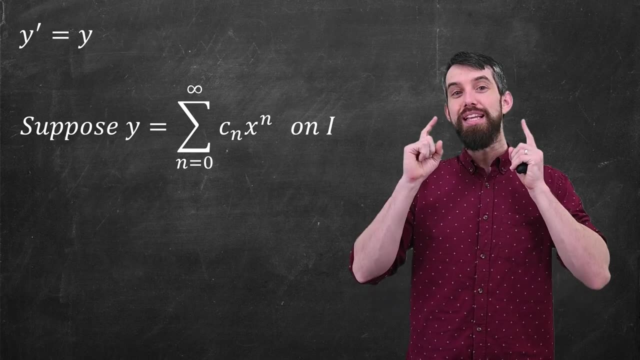 of things. Does that add up to a finite number or does it diverge? So what I'm going to do right now is make an assumption that I haven't justified, but an assumption right now that this does have a convergent power series on some interval. i Now, before we jump into solving this differential, 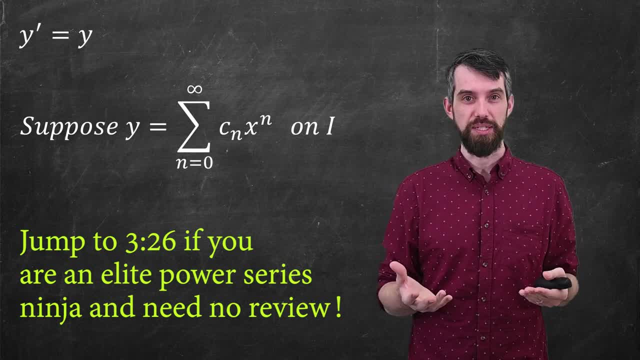 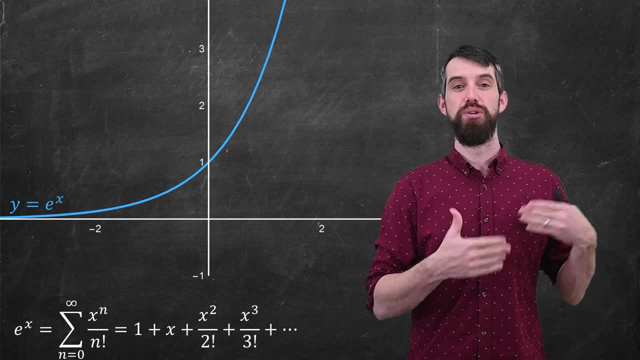 equation. I want to review just a couple important facts about series. First thing I want to talk about is how we use series to approximate functions. My claim here is that this is the power series expansion for e to the x: about x equal to zero. And if I look at 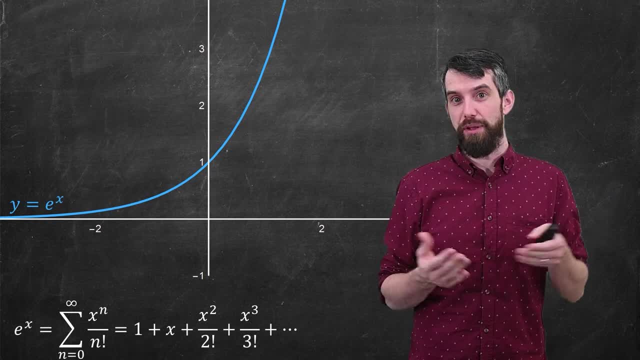 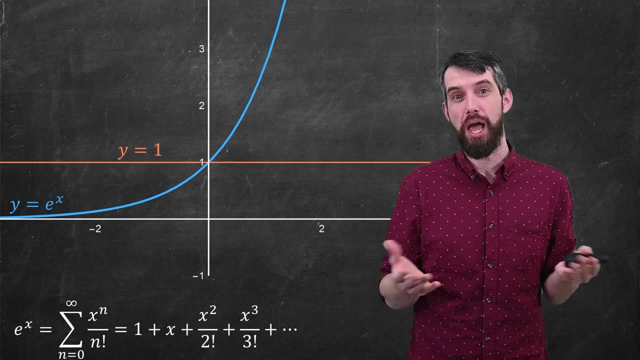 this sum. it's well a sort of infinite polynomial, if you wish. But if I only take the very first term, if I only take y equal to 1, then that's the graph of just a straight line. You'll notice that. 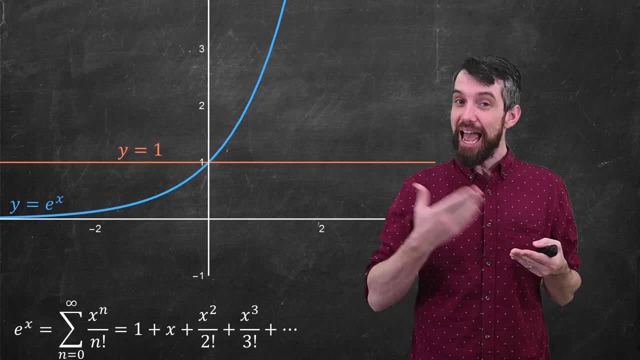 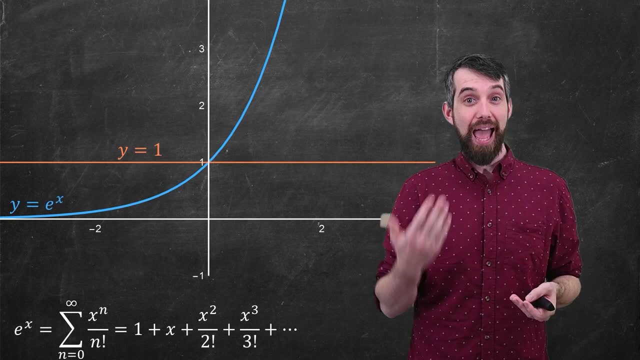 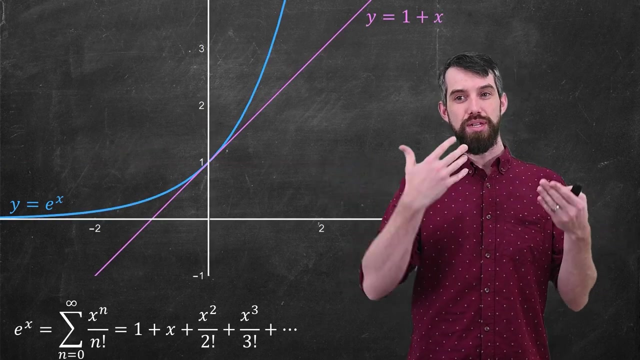 y equal to 1 is actually an excellent approximation to e to the x at the value of x equal to zero, but a kind of terrible approximation. 1 plus x, if I add the next term, is actually a better approximation. Now I get another straight line. but because it's now tangent to e to the x, 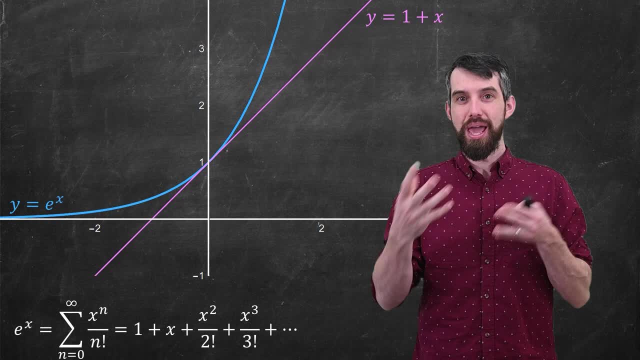 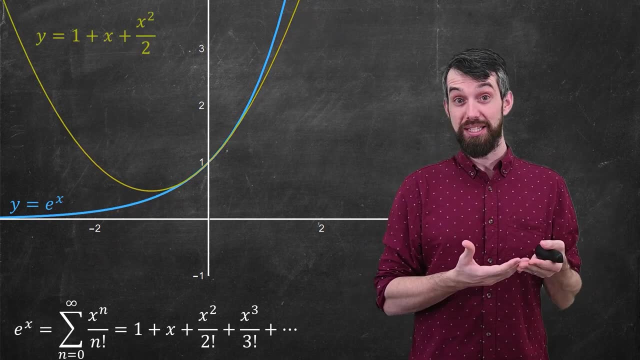 it's not only a good approximation at zero, it's sort of an okay approximation around zero. If I add now the x squared over 2 term, so I get quadratic. now you're starting to see that this quadratic lines up really nicely. with e to the x I could add a cubic term. it now lines up even. 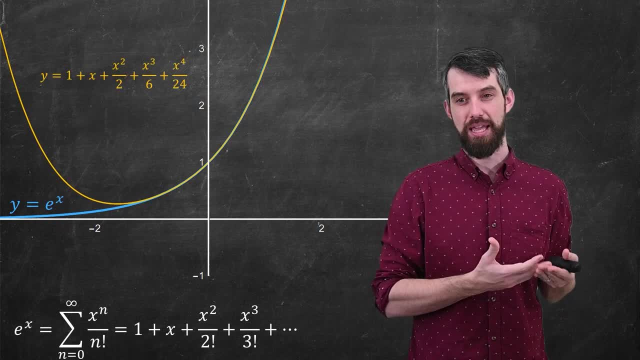 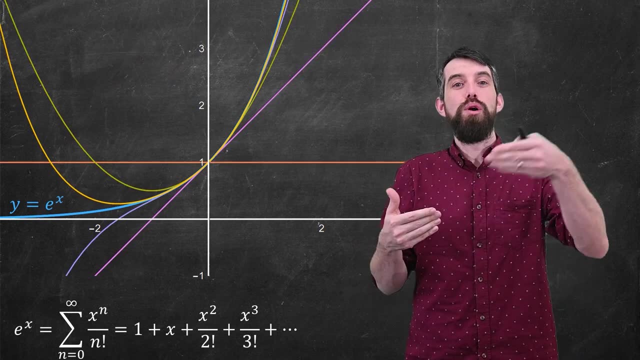 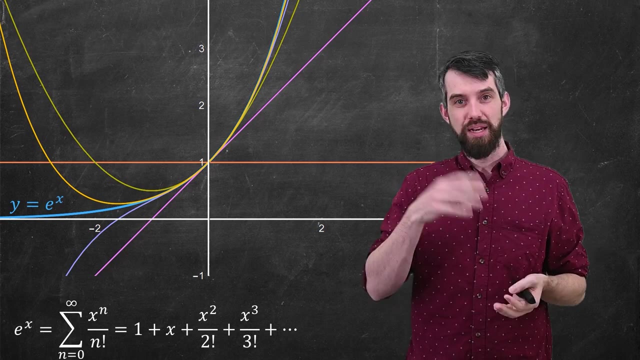 better. I can add a quartic term, it adds up better yet again. So here's the point: If I put all of those polynomials up here, as I have more and more terms in this series- expansion, I get a better and better approximation for e to the x. It's in this sense that we think that 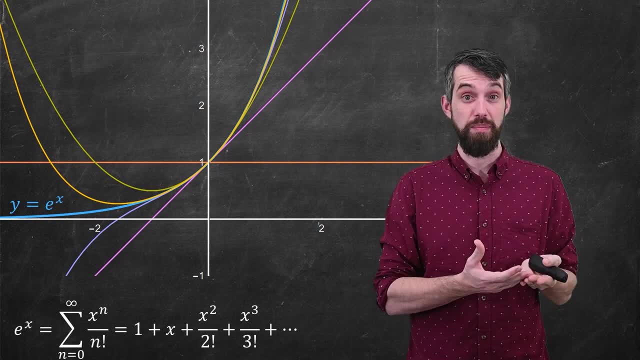 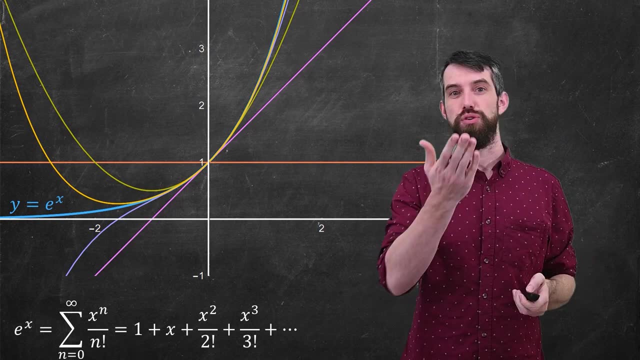 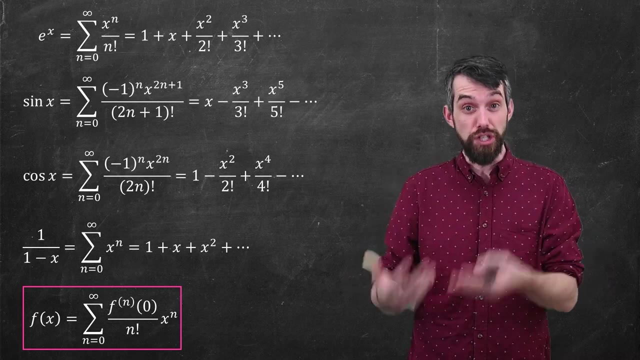 e to the x and this infinite series are the same thing because they converge to be the same thing, as the number of terms you take goes to infinity. The next thing I want to remind you of is the expansions for a lot of the standard functions, like e to the x, sine cos and the geometric 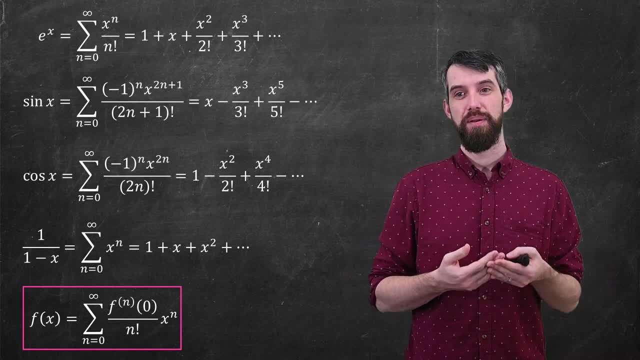 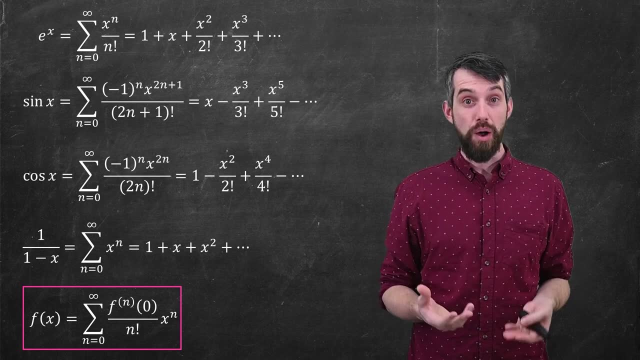 series which adds up to 1 over 1 minus x. So these are all known series and we're going to use them as we solve differential equations. Now, the way these came about were that they were Taylor series centered at the value of zero, or sometimes called Maclaurin series. Either way, they came from this. 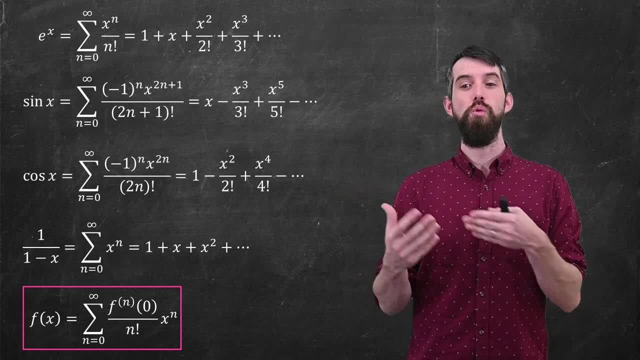 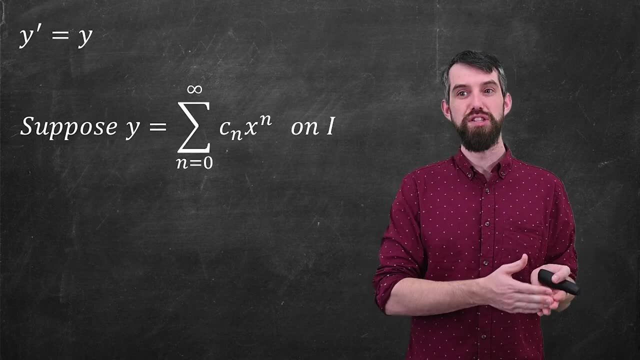 formula highlighted at the bottom, Namely, if you can compute a whole bunch of derivatives and see some nice pattern, you can get the series out of it from there. All right, let's get started. All right, so let's return to the differential equation that we were studying and the 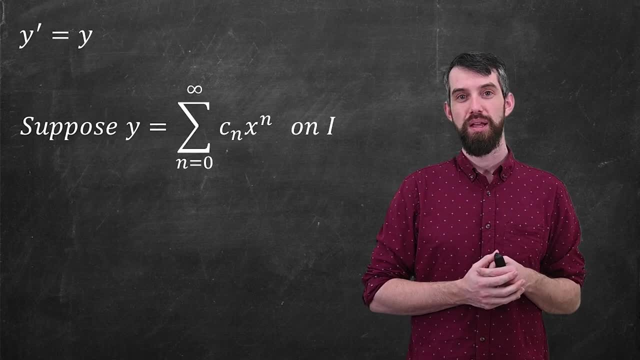 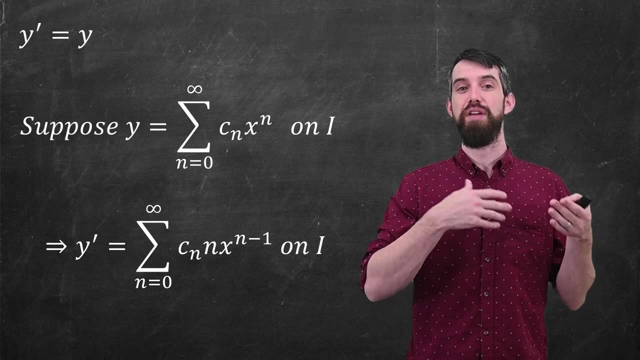 assumption that it can be written as this convergent power series. The first thing I want to do to that assumption is I want to take its derivative. Indeed, we have a theorem that says: if you have a series which is convergent on some particular interval, you can take what we 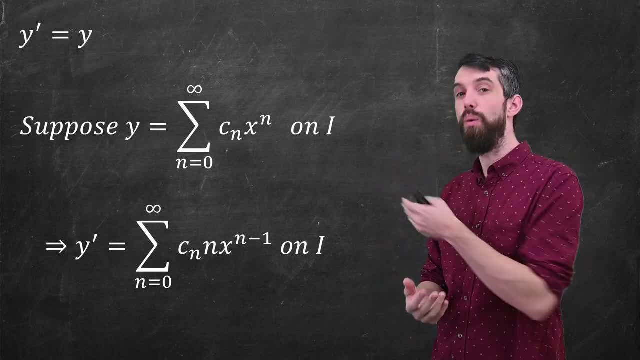 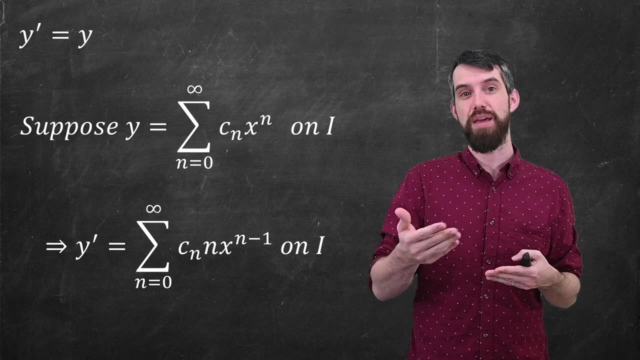 call the term by term derivative of it, which is what I've done here. So the sum stays out the front and then for each term I take that derivative: x to the n goes to n, x to the n minus 1. When you take this term by term derivative, you get that it's also convergent on the interval i. 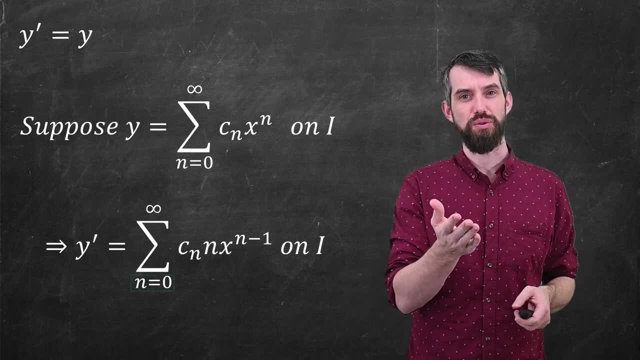 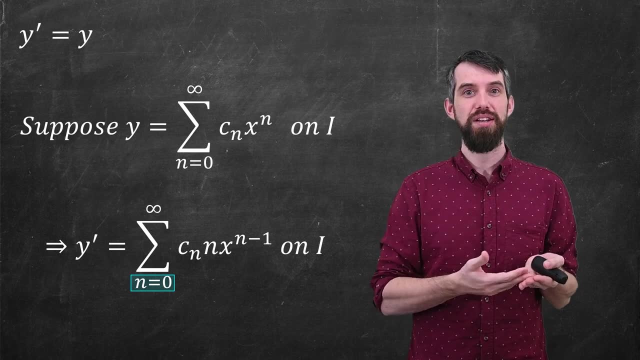 I'm going to do one little trick here. Notice that there's actually a zero on the bottom, n equal to zero. But if you plugged in n equal to zero, there's also an n in the expression here- cn times n. So when you plug in n equal to zero, you just get a zero term, So having n equal to zero. 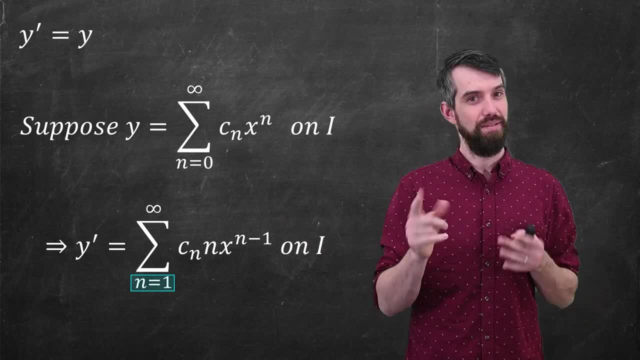 doesn't do anything, So I'm just going to just replace it with the value of 1 instead. You'll see why in a moment. Nevertheless, I have a y, I have a y prime. The claim is that y and y prime are equal. 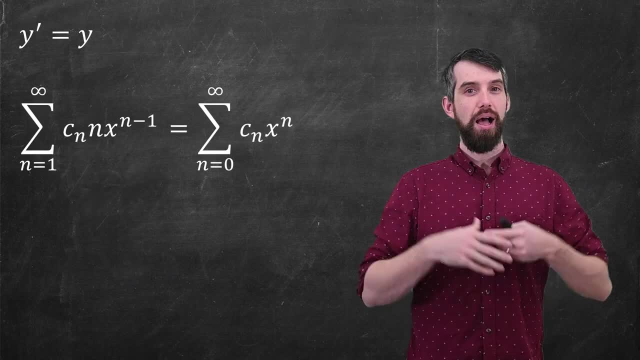 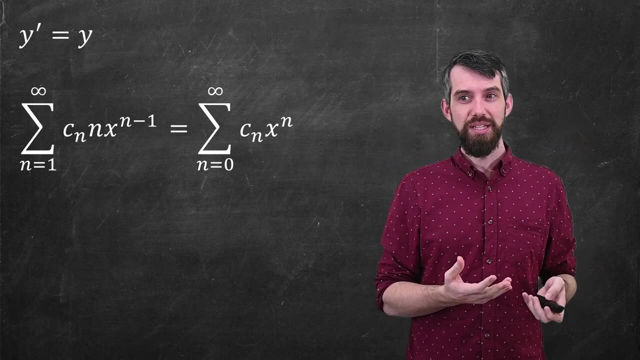 so let me just plug those two things equal to each other. I have two series. I want to compare them, I want to compare the coefficients, but I unfortunately can't quite do that. The reason is that one is coefficient times x to the n, but the other 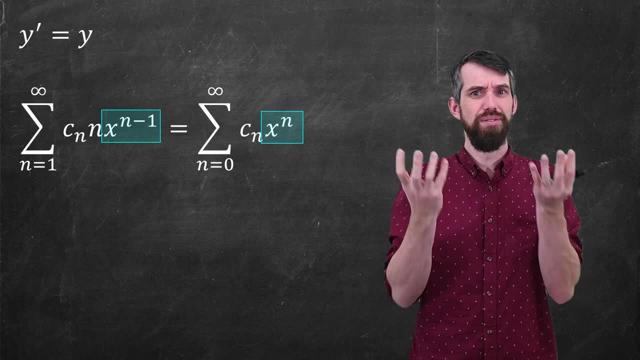 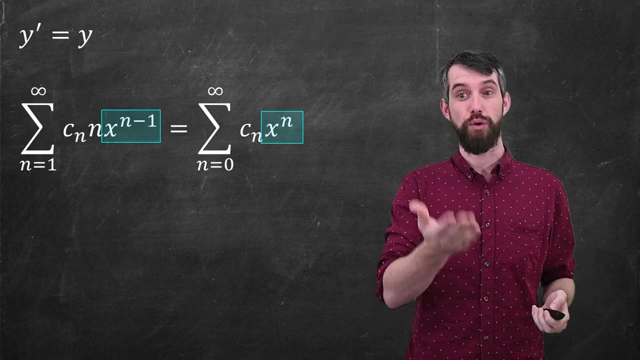 is x to the n minus 1.. That is, they're not written with the same index. but that's okay. We can shift index on series like these. For example, we can send n to n plus 1.. This is just. 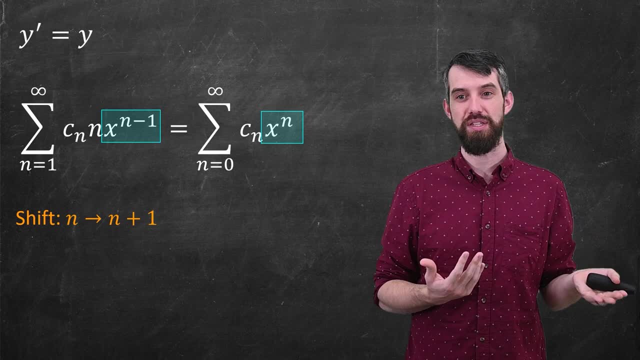 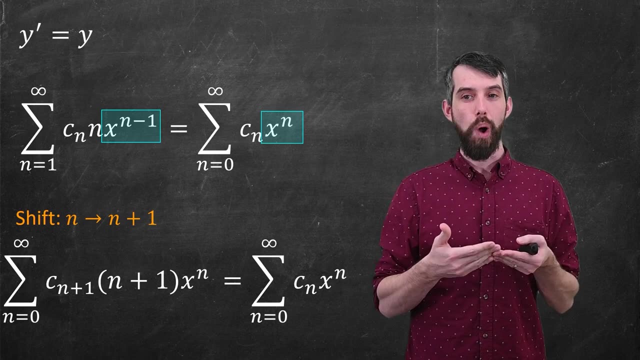 just rewriting our sort of indexing variable that keeps track of this series, So we're allowed to do this kind of shift. So if I do that, several things happen. Instead of starting at n equal to 1, when you shift n to be n plus 1,. 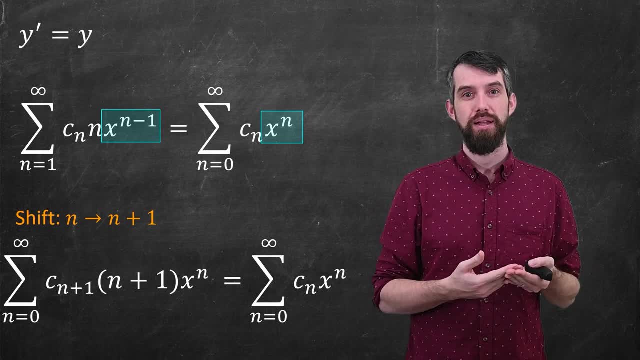 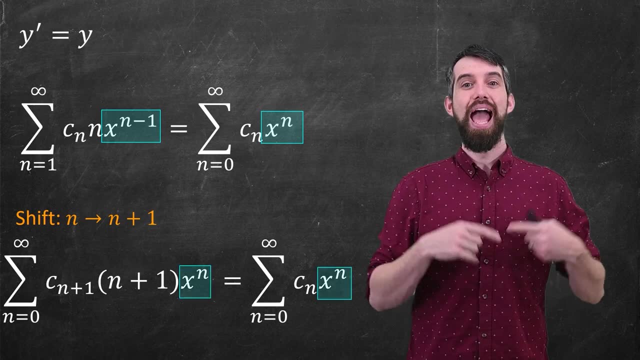 that's now starting in the new index at n equal to 0.. Instead of cn, it's cn plus 1.. Instead of n, it's n plus 1.. And now the good part, which is the exponent, the x to the n. 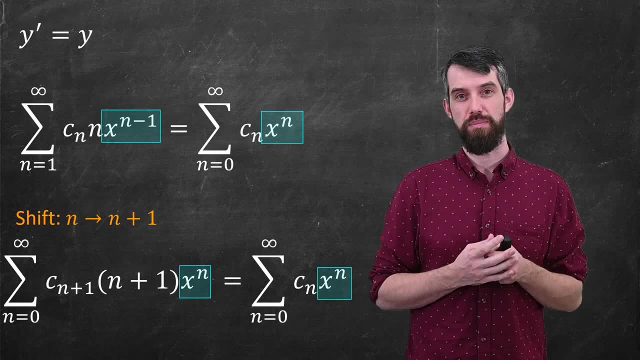 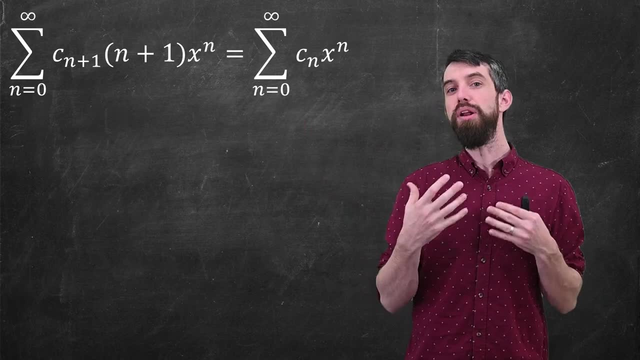 minus 1 turns into an L and x to the n. And now I do have like terms. They are the same on the left as it is on the right. They're coefficients of x to the n. Okay, so, clearing some space, I'm now going to use an identity theorem, And it says that: 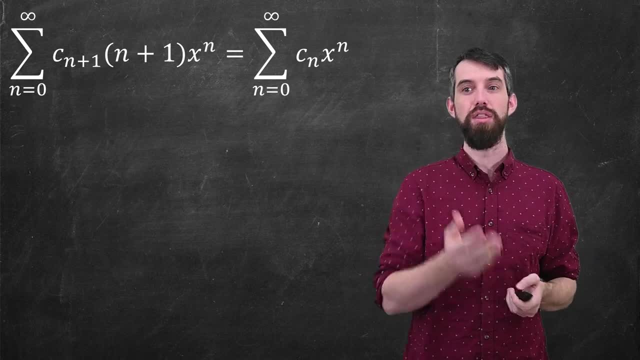 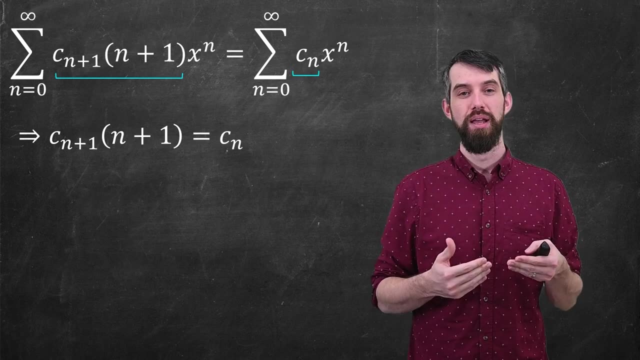 if I have x to the n on both sides, then if I look at those coefficients, the things in front of the x to the n, they must be the same And this gives me the equation that cn plus 1 times n plus 1 has to be equal to cn. It is often 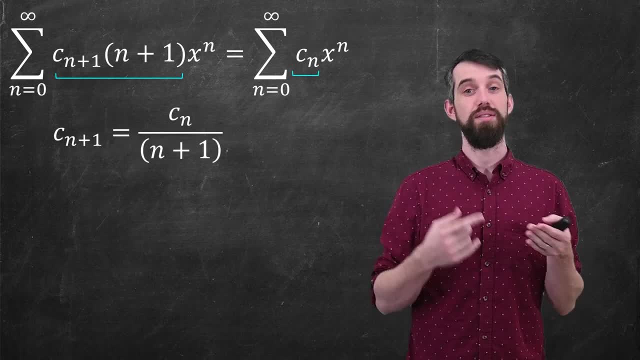 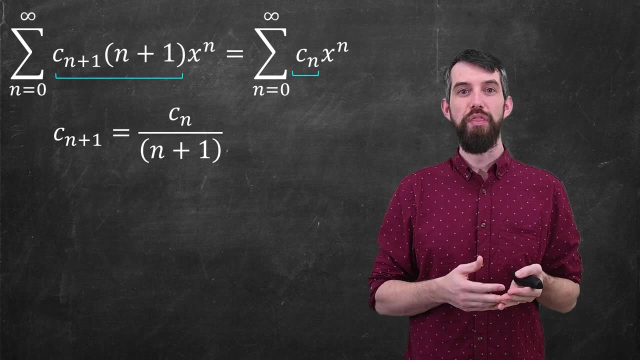 convenient to rearrange this equation and say that cn plus 1 is cn over n plus 1.. What I have here is something different than what I have here. What I have here is something called a recurrence relation. It tells me what the n plus 1th coefficient is in terms 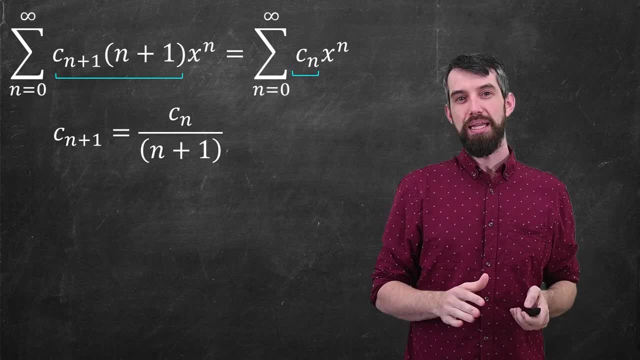 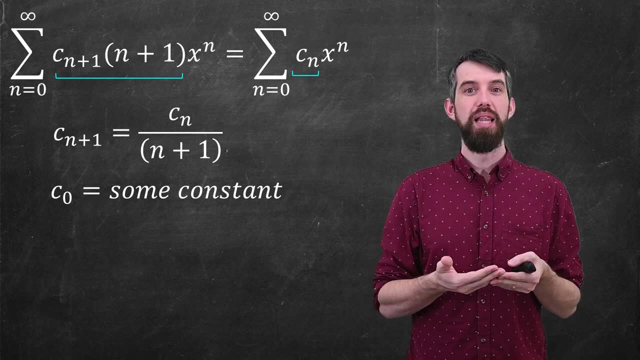 of the nth coefficient, For example. let me assume that c0 is just some constant. I'm not going to try to solve it, It's just a constant. c1 would be like plugging n equal to 0 into this formula. In other words, what the c1 would be would just be the value of 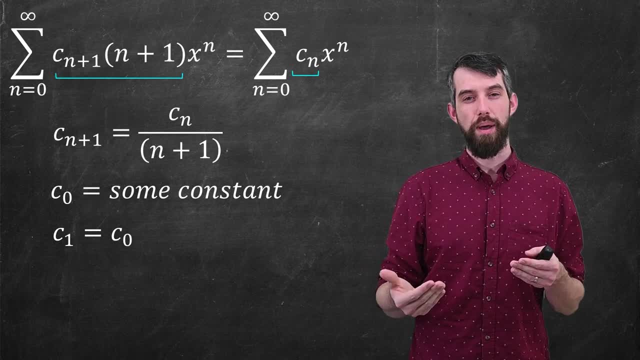 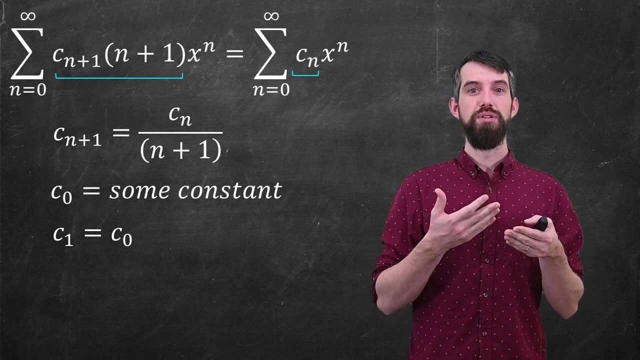 c0.. In other words, c0 on the top and 0 plus 1 on the bottom. Okay, great. So now I figured out the c1.. What about the c2?? Well now, c2 is like using n equal to 1.. So it's. 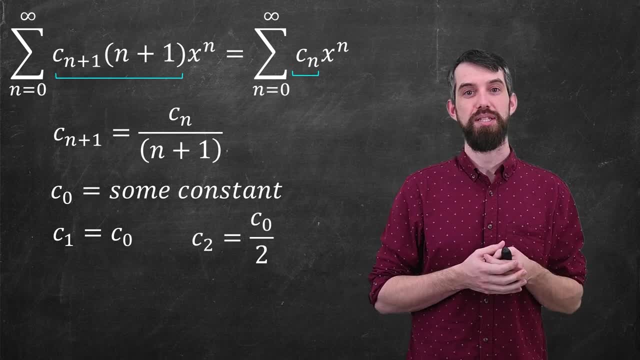 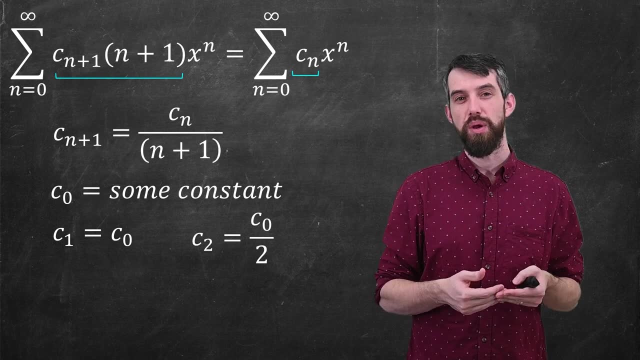 the value of c1 on the top, which we just saw was the same as c0, and then divided by 1 plus 1 is 2 on the bottom. Okay, so this is c0 divided by 2.. What about c3?? Well it. 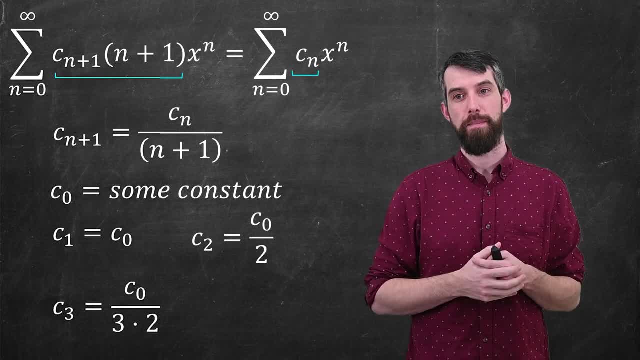 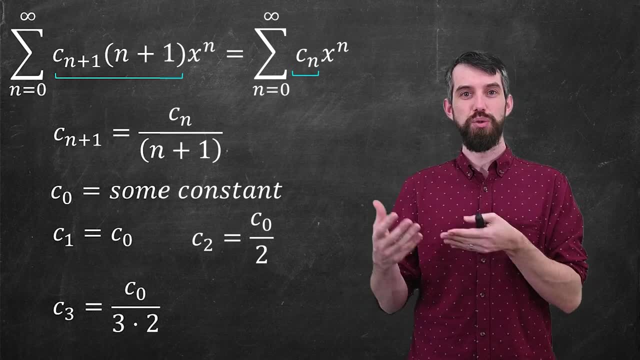 would be that thing: c0 divided by 2, but then divided by 3 on the bottom. What about c4?? Well, it would be c3 divided by 4, and so on. So what this recurrence relation is doing is it's starting with c0 and then dividing. 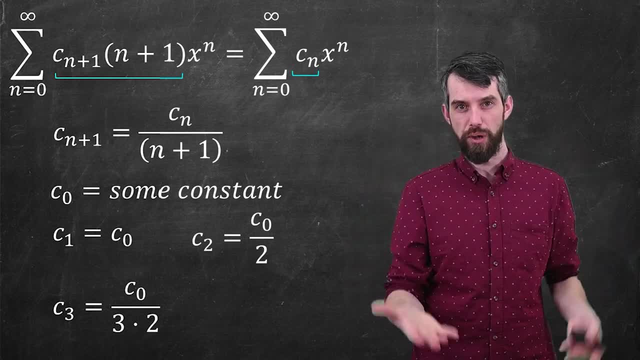 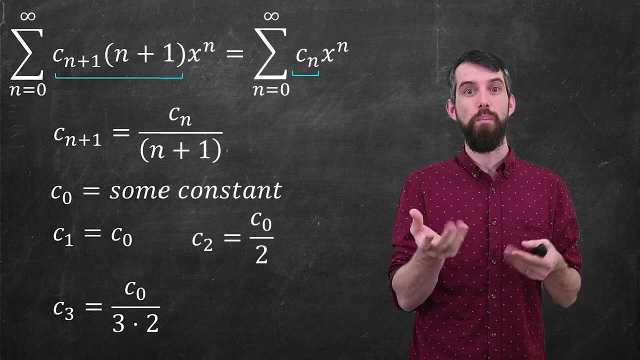 it by 1,, then 2,, then 3,, then 4,, then 5,, then 6,, and so forth, And so generally I'm going to say that cn, the nth term, is just going to be the initial c0, but divided by n, factorial. 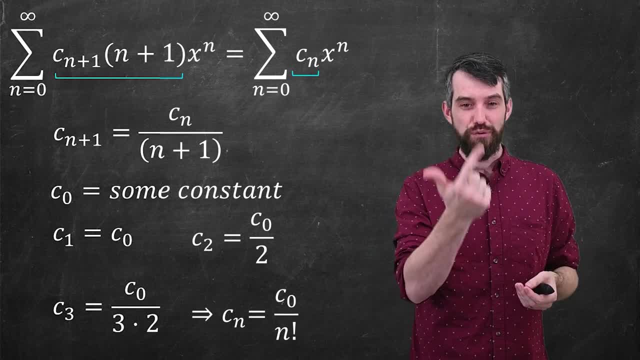 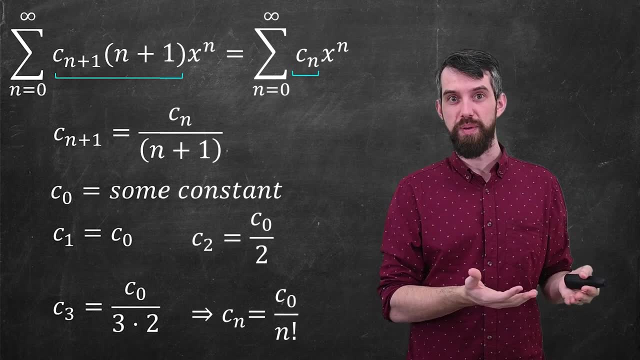 For example, c5, say, is c0 divided by 5 times 4 times 3 times 2 times 1, which is 120.. Okay, so we knew what the general expression for y was supposed to be, but now we've solved. 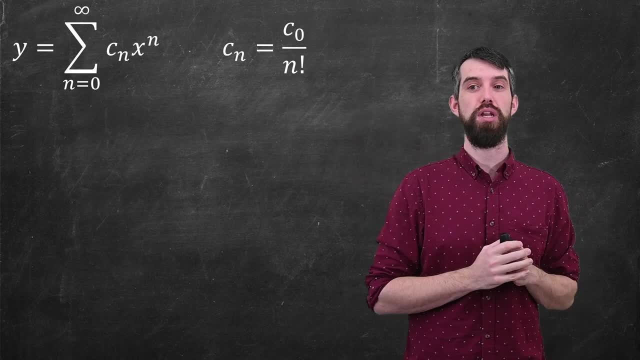 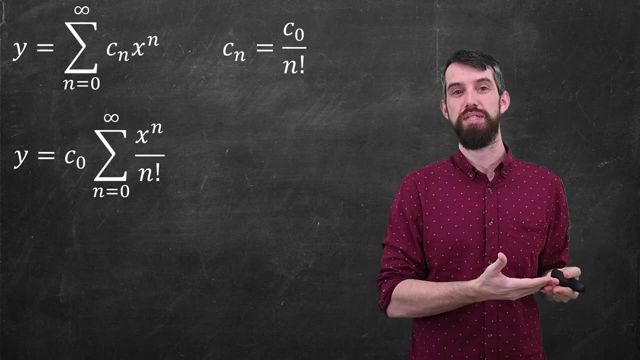 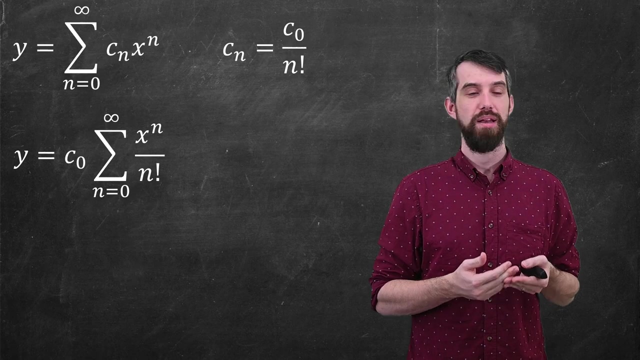 for the cn's. So let's go back together and say I've got my general solution: cn x to the n, and I know that the cn is c0 divided by n factorial, and so my final answer is thus: y is a constant times the sum of n equal to 0 up to infinity. x to the n over n factorial. Now this is precisely: 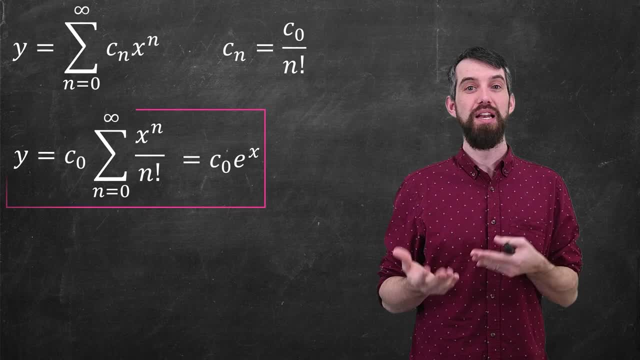 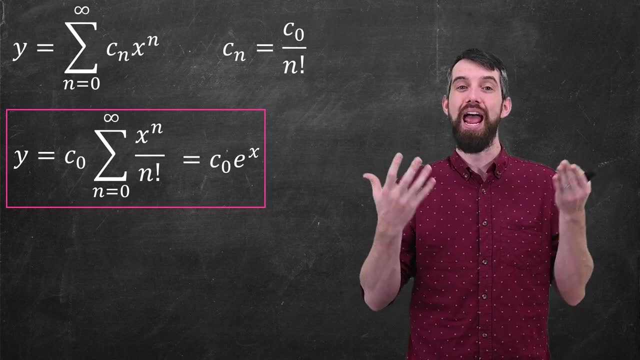 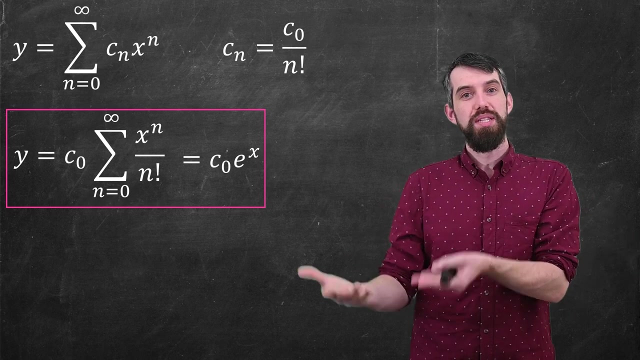 what we saw: the expansion of, That's just the expansion of e to the x. It's a constant times e to the x, And so we have recovered the same solution that we had at the very beginning. It's worth noting here that when we tried to solve for the cn, we determined all the 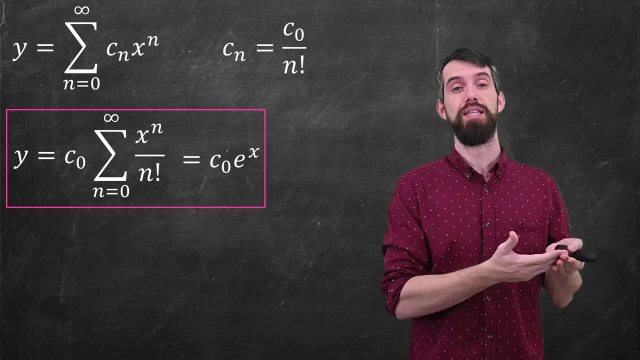 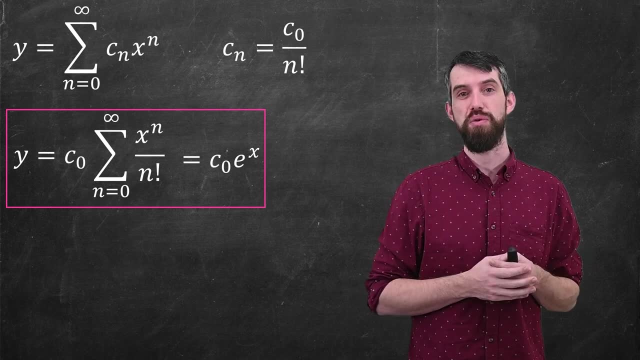 cn's in terms of c0, but we never determined what the c0 itself was. If I had specified an initial condition, then you could have used that, plugged it in and then gotten the value of c0.. By the way, mathematicians often will define e to the x in different ways. It's not incorrect. 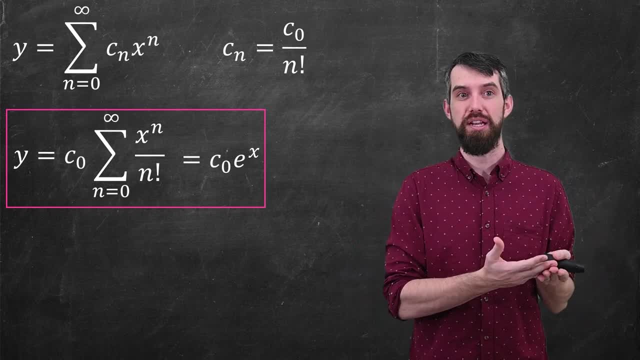 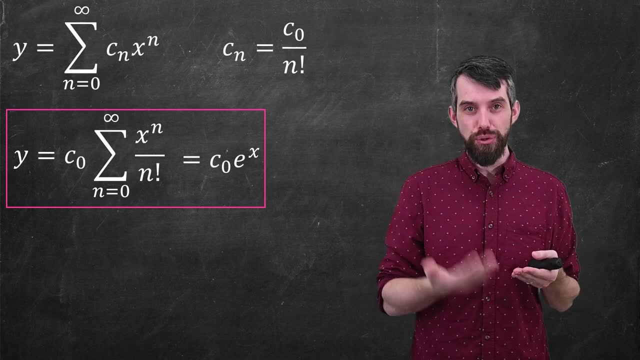 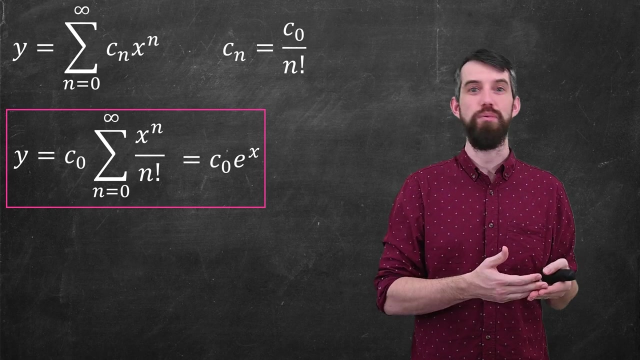 to define e to the x as the power series. Like what is this function, e to the x? The answer is: it is that power series. Mathematicians say that e to the x is the solution to the differential equation y prime equal to y. Perhaps, with the initial condition, the y of 0 is equal to 1, which will impose 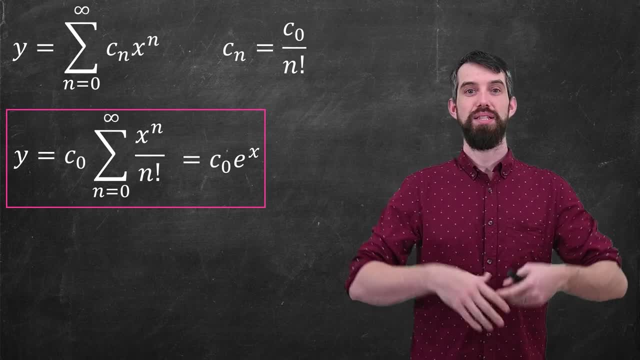 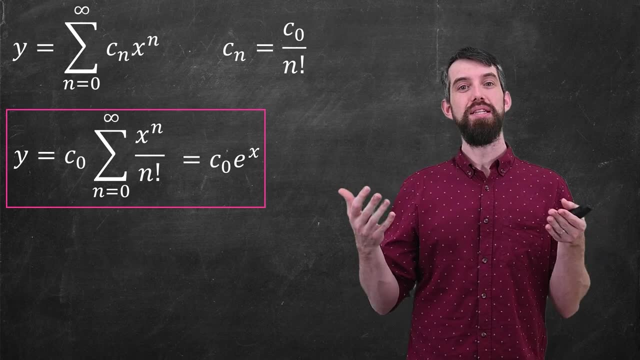 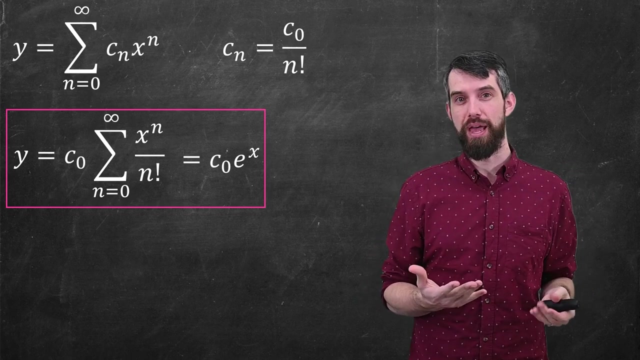 that the constant c0 is just equal to the value of 1.. Nevertheless, these competing definitions are aligned in this particular methodology. The final thing I want to talk about is when does a series like this converge? Now, e to the x is known to converge everywhere, but how do we know that? There is a theorem that 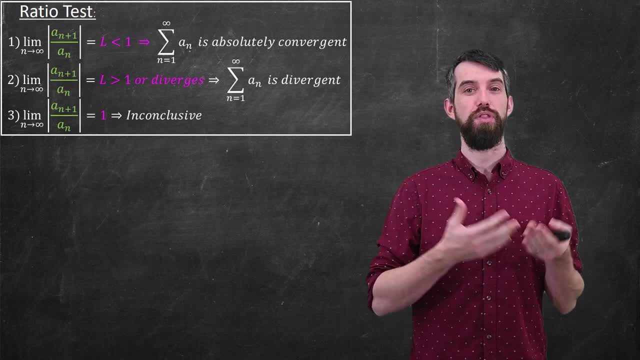 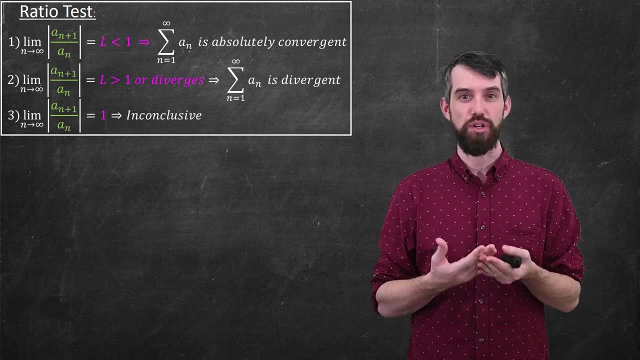 I will remind you about from back in first-year calculus, called the ratio test. It says that if you have some series, some sum of a n's- now where, in our case, we're thinking that the a? n's are probably a constant times- an x to the n, but nevertheless just some series- 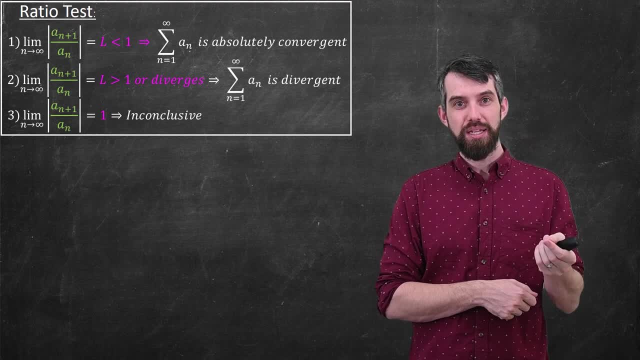 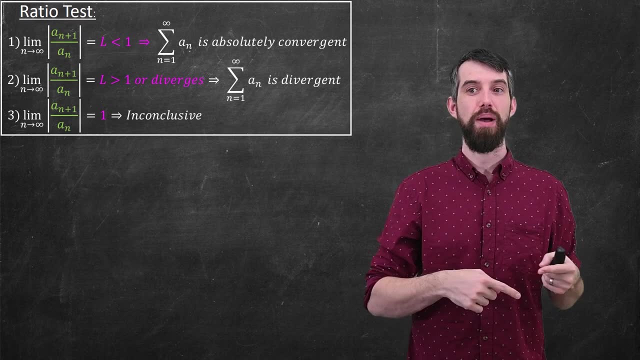 in general, then what you do is you look at the limit of the ratio with successive terms: a n plus 1 over a n. You get a couple different possibilities. That limit might be less than 1.. That limit might be less than 1, in which case the test tells you that it converges. 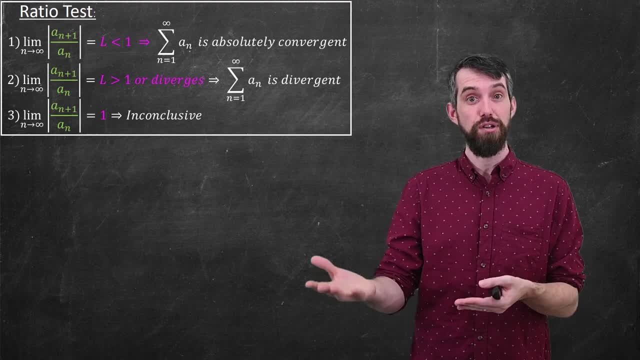 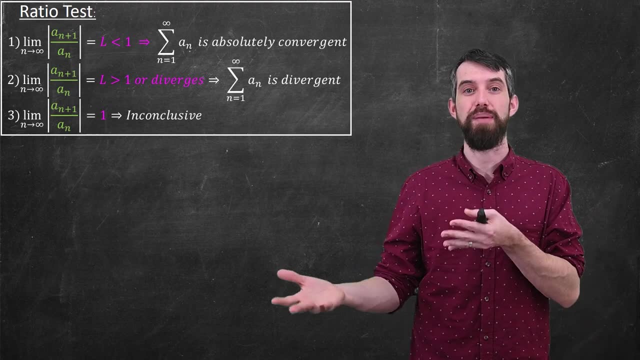 limit might be greater than 1, in which case the test tells you it diverges, or that limit might be equal to 1, in which case, unfortunately, the test fails or is inconclusive and you're gonna have to do some other types of analysis. So let's. 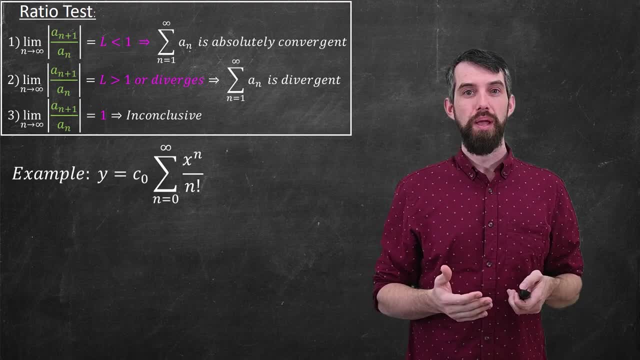 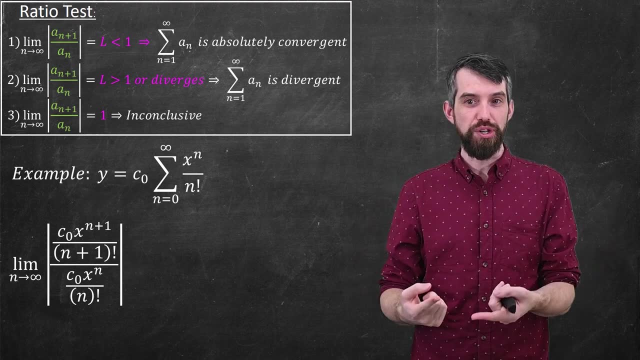 see this for our specific example of e to the x. So if I take that ratio I'm taking a limit as n goes to infinity. on the top, a n plus 1th term looks like: well, the constant x to the n plus 1 over n plus 1 factorial, That's the a n plus 1. 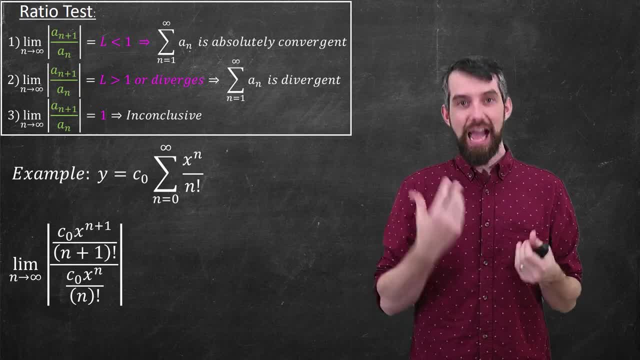 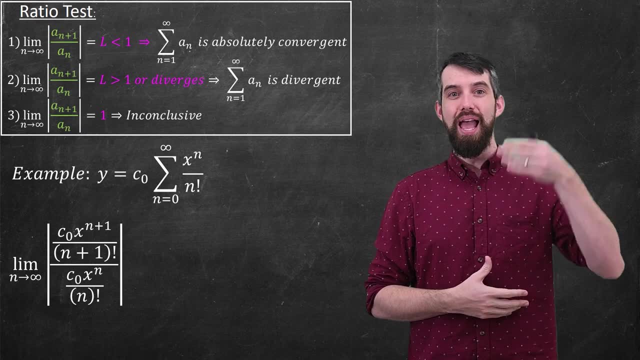 on the top, On the bottom, very similar. there's the c? naught, there's the x to the n and the n factorial. Now, a lot about this messy expression cancels the c? naughts, cancel the x to the n plus 1 on the top and the x to the n on the bottom. 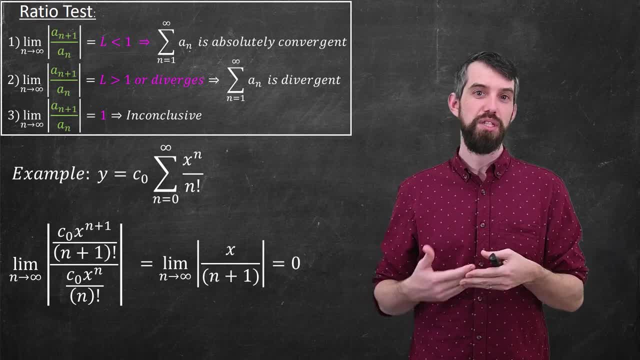 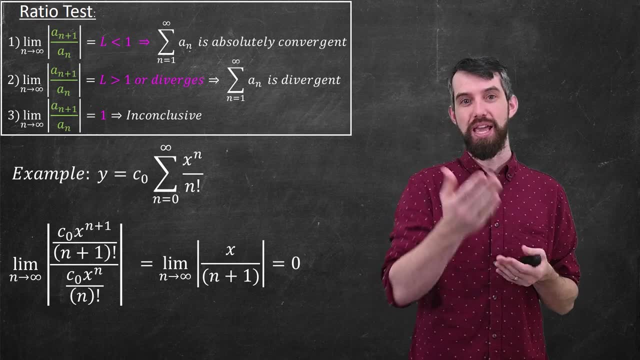 they mainly cancel. they leave you just 1x. Likewise for the factorials. if you have n plus 1 factorial on the bottom and n factorial on the top, almost all of n plus 1 cancels from the n factorial and just leaves you with n plus 1 on the. 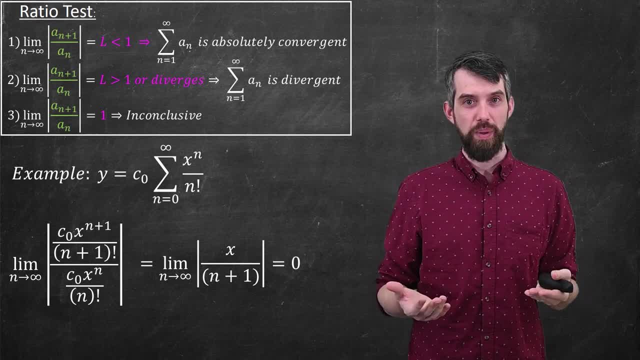 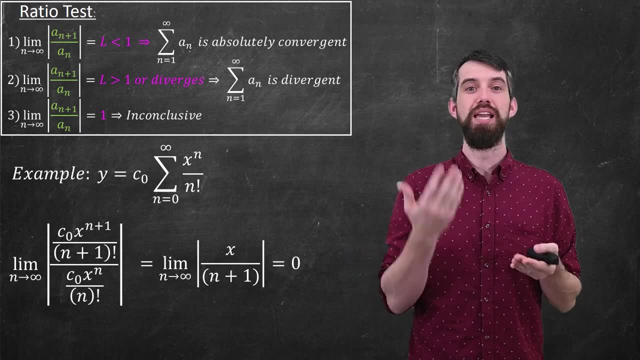 bottom, This expression that we have is going to be 0, because no matter what your value of x is, say a billion, then you can always find values of n large enough to take x divided by n plus 1 to as small as you might wish. So 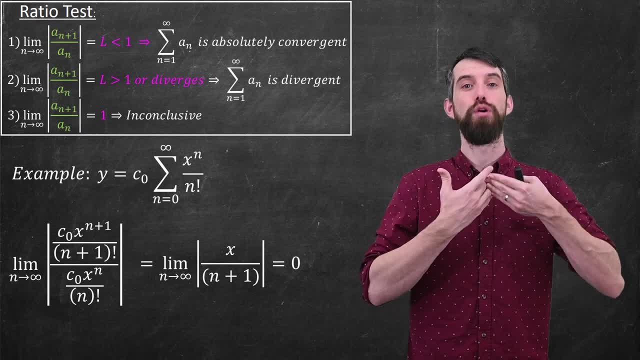 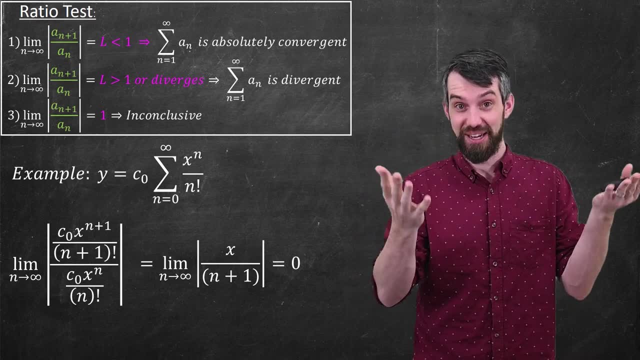 this limit is 0 and thus, by the ratio test, it converges for all values of x. Now, this video is just the first on a series of videos about, well, series, a list of videos about series, perhaps would be better to say. Nevertheless, we're going. 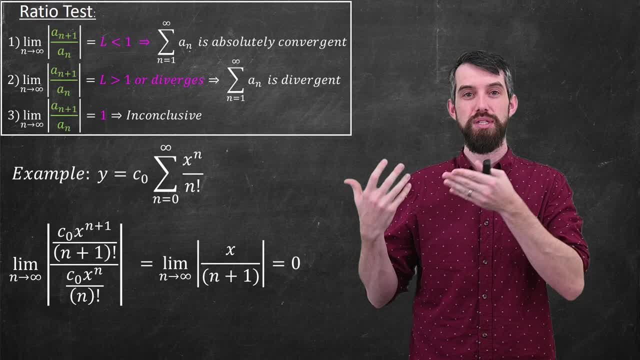 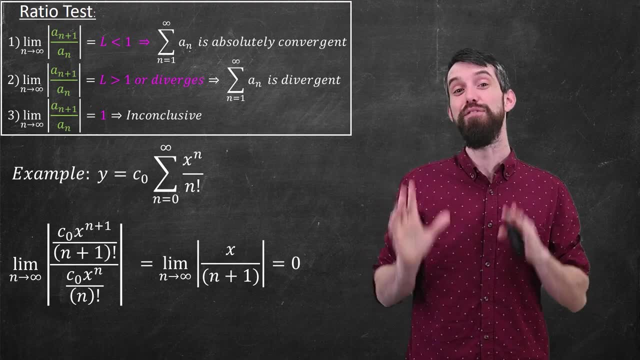 to talk more in more complicated situations about how you can use series to solve differential equations over the course of the next couple videos. So I would encourage you to subscribe, give this video a like if you enjoyed it, and we'll do some more math in the next video.